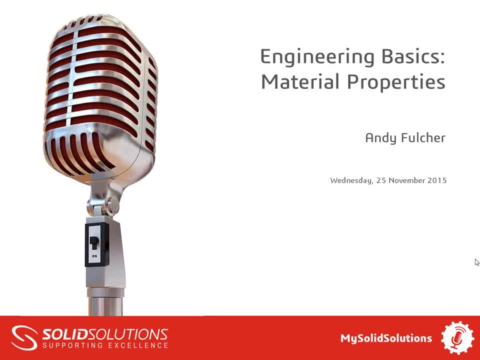 Welcome to Webcast Wednesday. My name is Nick Sibley, I'm producing this morning's webcast, and sat along beside me is Andy Fulcher. He's going to be taking us through engineering basics- material properties. So without further ado, I'll hand you over to Andy. 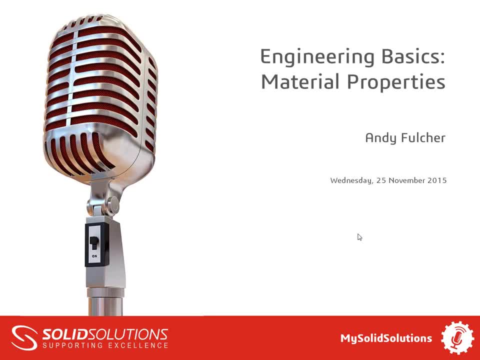 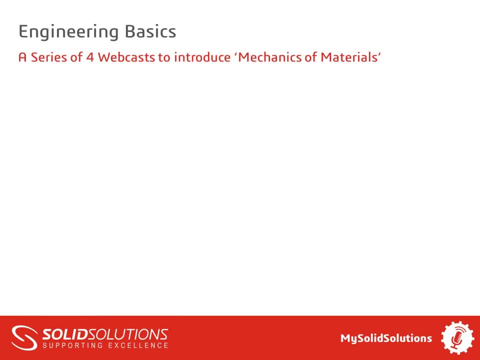 OK, cool, Nick. Thank you very much. Good to be with you again. This is a series of four webcasts- We did two last Wednesday and I've got one more to do this afternoon- Introducing the topic of mechanics of materials, which is a basic topic which you would typically study, maybe at an undergraduate level of mechanical engineering. 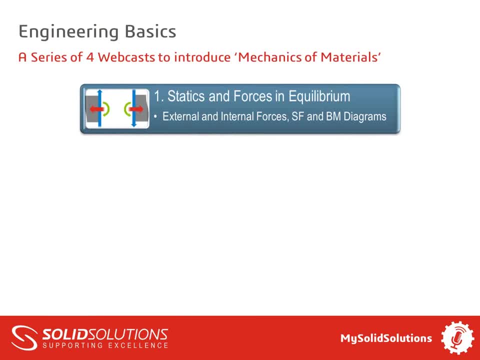 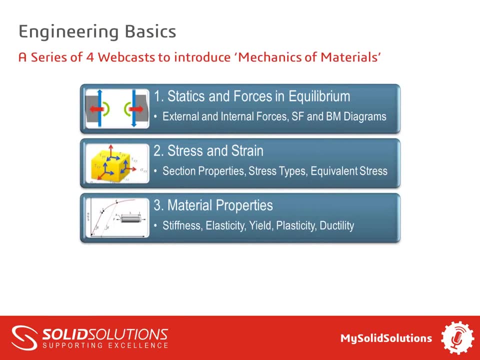 Last week we looked firstly at statics and forces in equilibrium. We then went on to look at stress and strain. Today we'll be looking at material properties, and then this afternoon we'll kind of be bringing it together and drawing some conclusions on how we might evaluate failure. 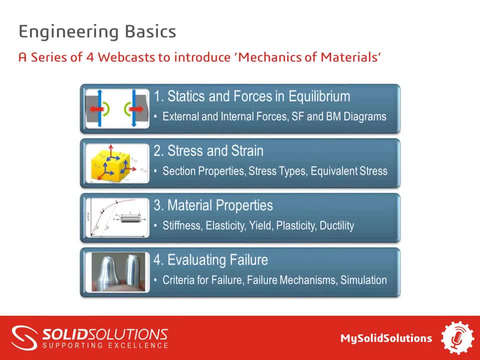 This is a logical sequence. If we want to understand how our parts perform in the real world, then we have to understand all these topics. We can't kind of get to the fourth topic, knowing how things will fail, unless we understand something about the previous three. 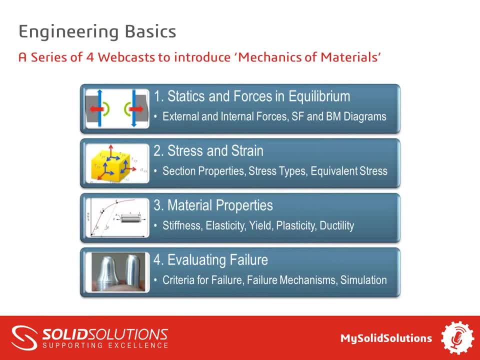 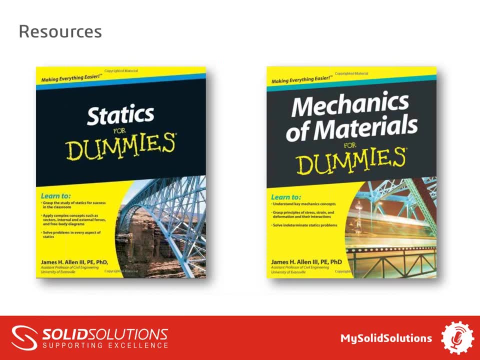 So today it's material properties. Just to show you the couple of books which I'd strongly recommend. I've bought these. In fact I bought these back in the summer and I've read them. They are both good and cheap, which I guess is a good combination. 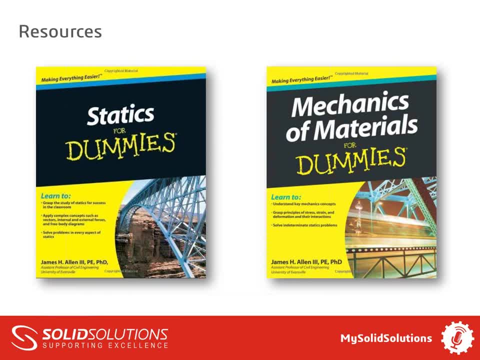 They're about $14.99 off Amazon. I don't get a commission on these. I'm not the author, but the guy who is explains some of these important topics extremely well, And both- the All four of the webcasts in these little mini-series kind of rely on the information covered in these books. 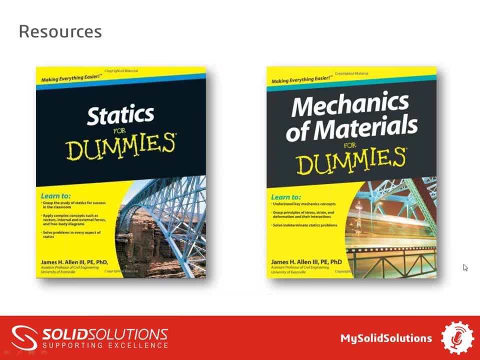 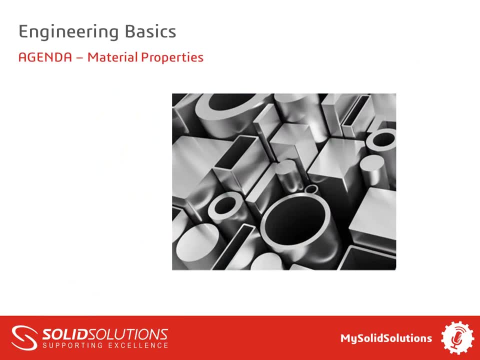 So statics first of all, then mechanics of materials, so I'd certainly recommend that you have a look at those. So today we're looking at material properties and various aspects of materials, So we'll be thinking about The very important properties of stiffness, elasticity, what it means to yield, plasticity, what actually makes 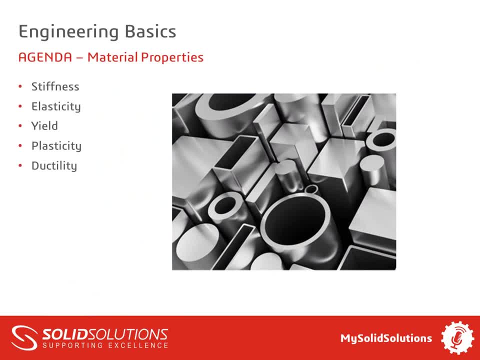 And of course saya is Hi, ductility and so on. these are kind of fundamental material properties. I should perhaps add a disclaimer in that you could do a complete three-year degree in metallurgy or material science, and they're clearly in half an hour or so. 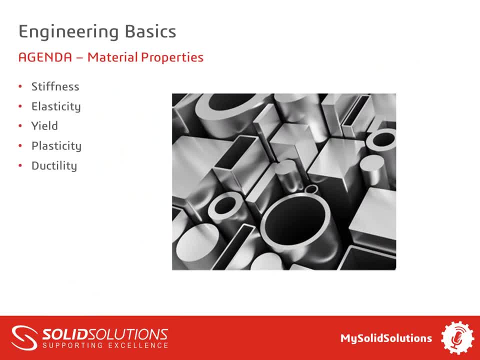 I'm not going to be able to cover a huge amount of detail, but I just want to give you the the flavor of what these topics cover, so that you're equipped then to either research further or or you know a bit more if you're coming to do hand. 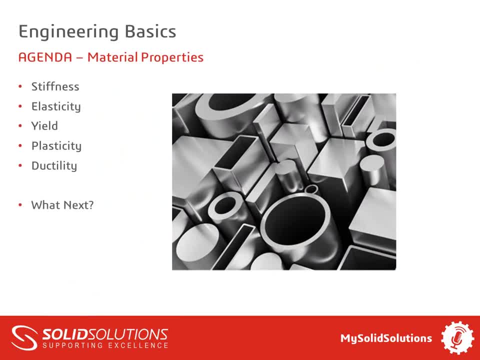 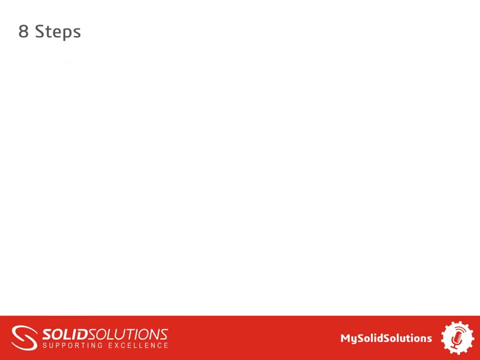 calculations or simulation studies on your own. I will finish off by kind of pointing to this afternoon and thinking about the failure modes. if you were here last week, you'll know that I've split my all my presentations down to eight topics. so I see these as eight kind of logical steps, eight things you need to. 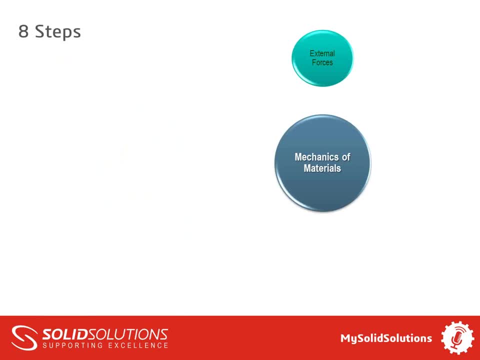 know if you can understand mechanics and material. and that starts with external forces, those forces applied to a apart or to an assembly by gravity, by working loads, by pressures maybe. and from those external forces we have to then turn them with those into internal forces. you have to see what the consequence in the material is of the 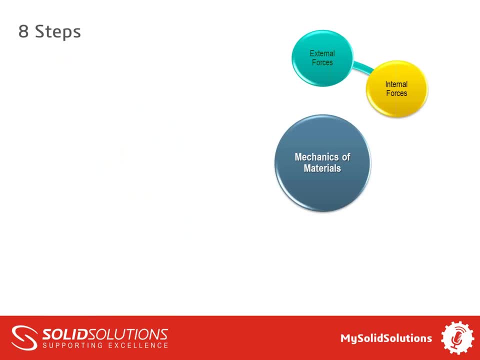 external forces and this will affect effectively boils down to three things as direct forces, shear forces and internal bending moments. once we've calculated those, we then need to determine section properties, because stresses are related to area. we need to understand section properties and you may recall, last week we looked at the simple section property of area. if we're 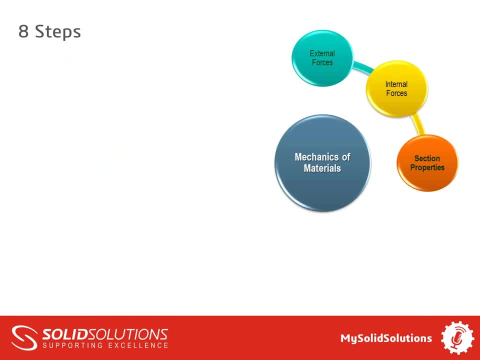 looking at direct or shear stresses. but if we're looking at things like torsion or bending, we need to understand things like the torsional constant or the second moment of area. which are they taking to get the material distribution on a on a cross-section? once we've got section properties and the internal forces, we 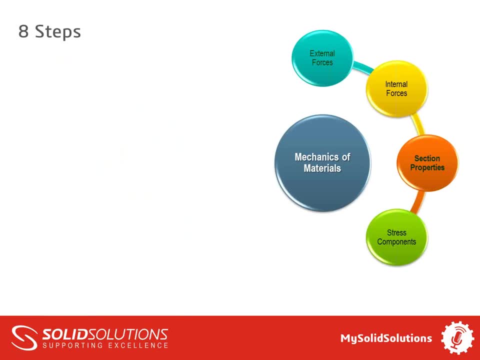 can then go and calculate our stress components by looking at the stress formulae, which might be quite simple in terms of a simple tensile stress over into a bending or torsional stress. it might be slightly more complicated but the those, those components can be calculated of. 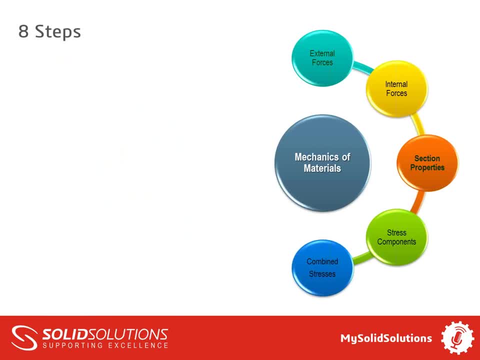 course, many structures are in complex stress states, so they will have maybe a bending stress and there may be an axial stress or a shear stress at all acting at the same time. so we need to know how to combine those and we looked at things like von Mises stress as a way of combining those. 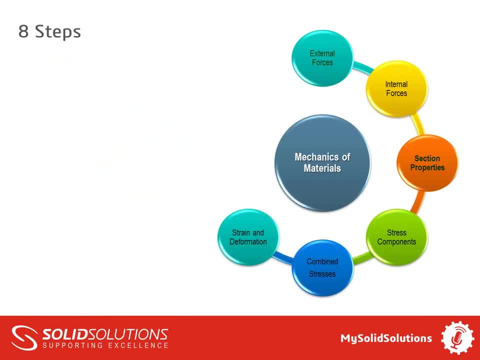 into an equivalent stress. we also touched on strain and deformation, how we calculate how much things will deform when external loads are applied, and that course leads us today. so everything we've done up to now leads up to this. this morning and this afternoon, and this morning we need to think about what 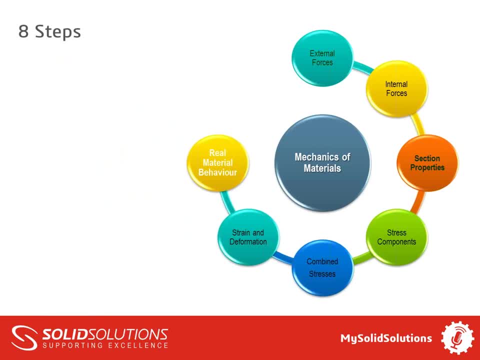 happens in real materials. how do real materials behave and and what properties in real materials do we need to calculate, or do we need to calculate or do we need to determine by experiment in order to then use the information we've we've calculated in order to make some sense of the stresses. 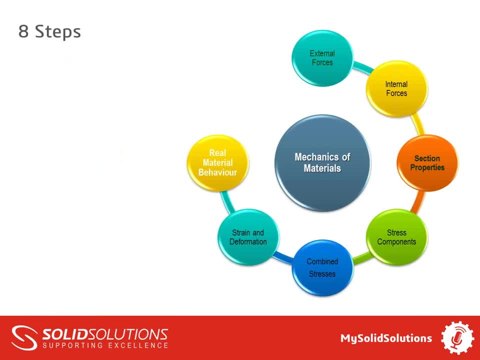 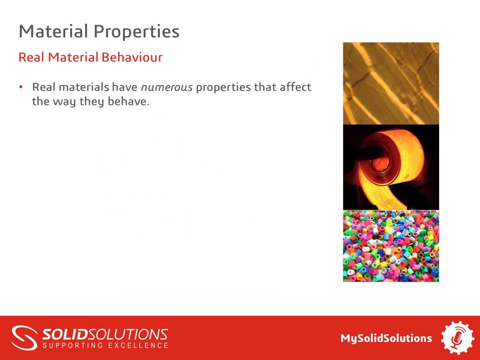 and indeed for deformation, to actually be able to calculate the deformation and then the self doing failure mode. so here are the. here we're up to step seven: real material behavior. real materials have numerous properties. I don't know whether there are dozens or hundreds of thousands, that certainly many, many 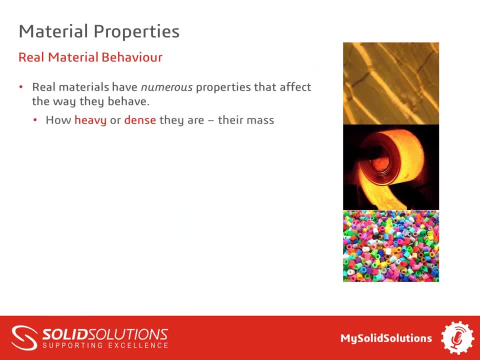 material properties. one material property is just how heavy they are or how dense they are. that will affect their, their mass, how hard or soft they are. many materials, or all materials in fact, will have a temperature dependency. so if we're looking at expansion- how much something expands or contracts- then 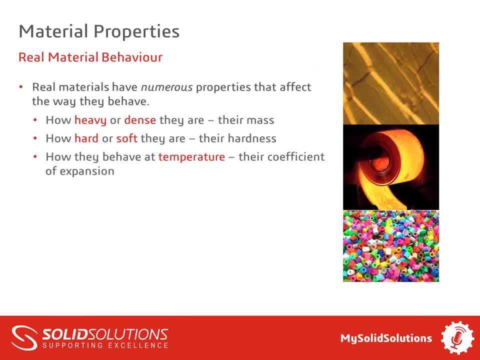 we'll need to understand how that babes at different temperatures, some materials, particularly things like these plastic bees here, they will be dependent on light or their environment, whether they corrode or not, and so on, and so on, and so on, and I'm sure you can imagine dozens of. 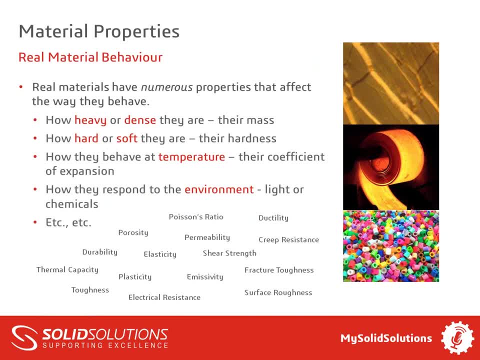 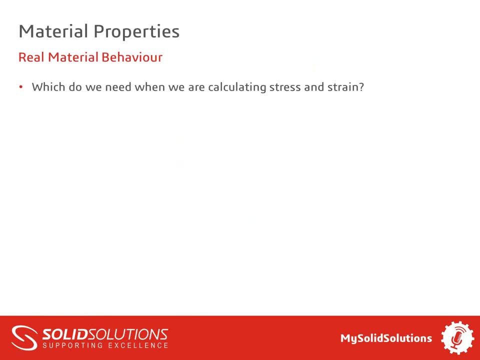 properties. I did a quick search on Wikipedia for properties of materials, and these are some which came up just immediately in a list. so the question then comes is, if we're working out stress and strain, what material properties do we need to know in order to do our calculations? well, here's a clue. 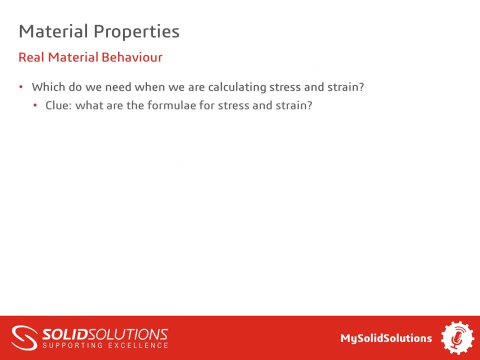 if we think back to last week, what are the formula we use for stress and for strain? here's a, just a simple illustration of a beam in bending, a force applied at the middle and two pivot points. and you may remember that the, the, the bending stress, which is a form of direct stress, is given by this formula. 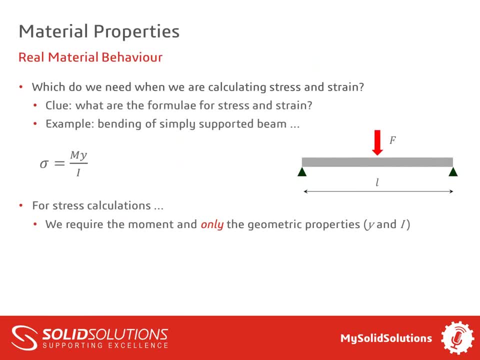 it's the bending moment times, the distance from the neutral axis divided by the second moment of area or the moment of inertia, the I property. notice that for calculating this value we don't need any material properties. it might come with a bit of a surprise. so if we're looking at a beam in bending, then 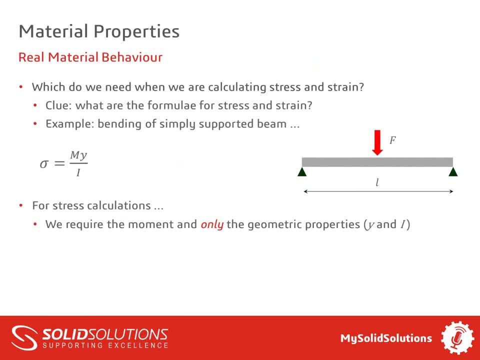 the stress will be the same whether it's made of aluminium or plastic or steel or glass. the stress will be the same. it only depends on the geometry and the the moment. similarly, if you're looking at a tensile stress in the cable, the stress is the force over the area and the stress, therefore, is the same whether it's 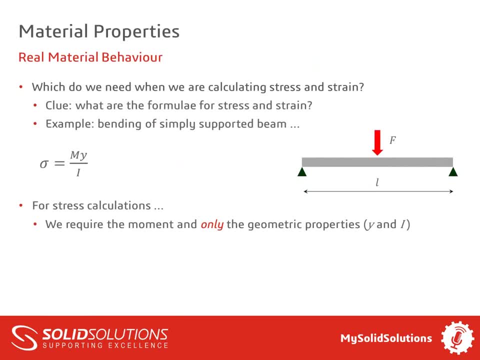 in a, an aluminium cable or a steel cable. when it comes to deflections, though, things are slightly different. here's a formula for the deflection of this particular beam. it's the load times, the span cubed, divided by the force applied by 48 EI, the, the, the L value and the I value, of course, again, material. 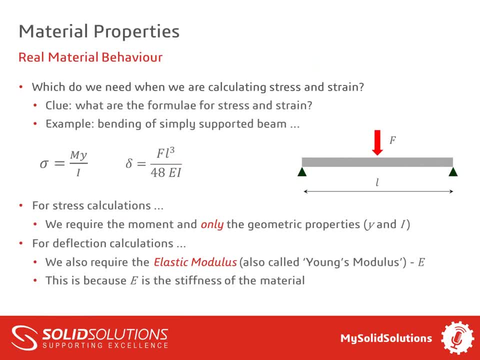 properties, but the E value is. the is a material property and it's the elastic modulus we would term. this is the stiffness of the material, the linear stiffness or the axial stiffness commonly known as Young's modulus as well. the elastic modulus and Young's modulus are the same thing. 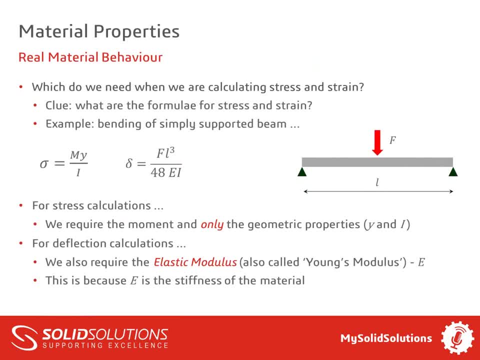 so if we make a beam out of aluminium, we make one out of steel, the E value for those materials will be different and therefore you'd expect a different bending amount to different bending deformation, even though the stresses would be the same. so the E value, the elastic modulus, is a crucial 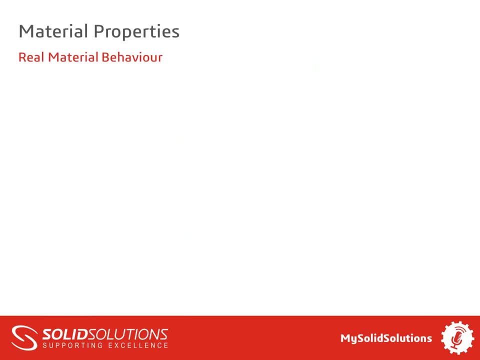 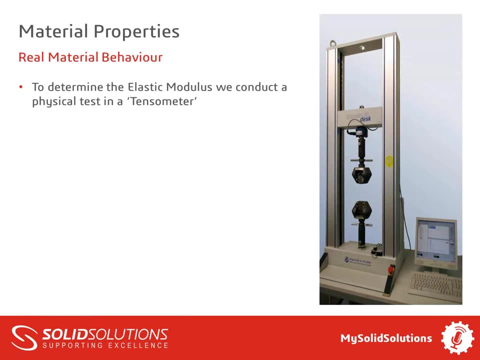 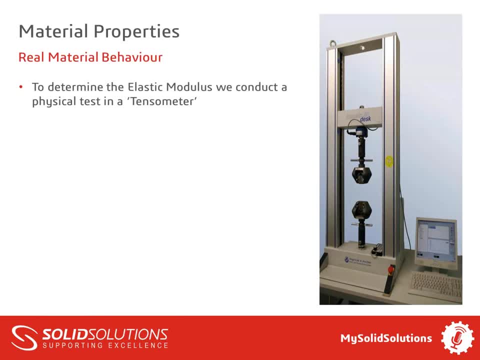 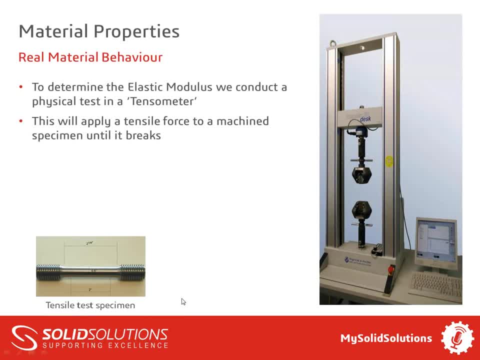 found of a typical test specimen. it's threaded at both ends makes it easy to wind into the jaws. it will be normally have a smaller cross-section so that it will fail, not in these threads, but it will fail through the middle. now this was exactly half an inch. 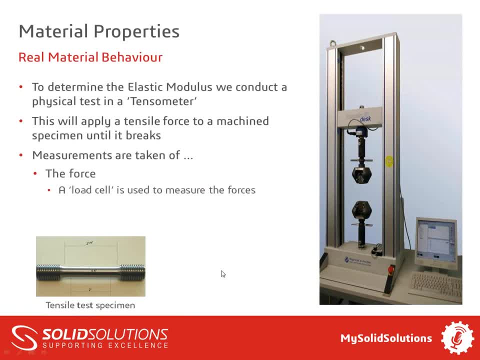 and then we take measurements of the force being applied to pull that test specimen apart. here you can see on the picture on the right there's a computer attached to this machine and you can see there's a graph and that will be plotting the deflection against the force. the force will be measuring a load. 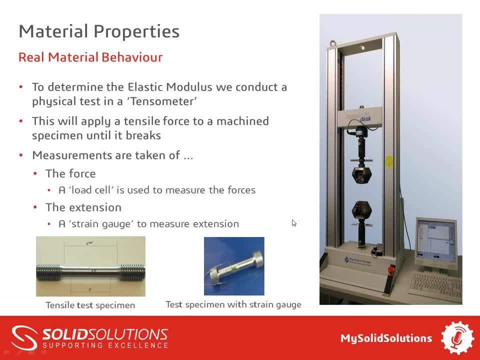 cell in the machine, the actual specimen, it itself will be stretching, and a strain gauge were used to measure the extension of that specimen. here's a small strain gauge applied to the specimen, some wires coming across. the strain gauge is an electronic device which will effectively- it's a Wheatstone bridge if you know your GCSE physics and 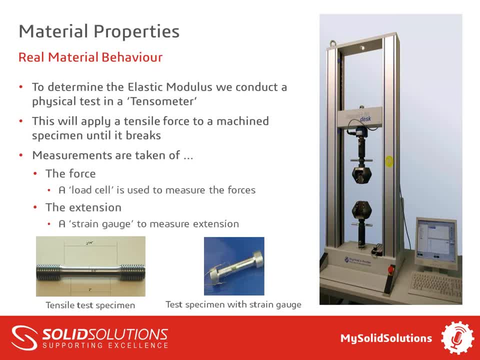 the current will vary or the electrical properties will vary according to the, the shape of material. so it's used to, it has to be calibrated but it then be used to measure the, the amount of deflection. we use something like this because it will be a very small deflection. it will be difficult to 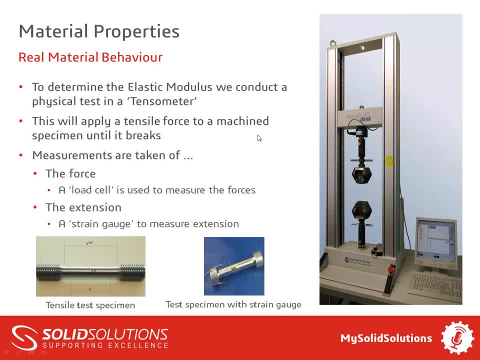 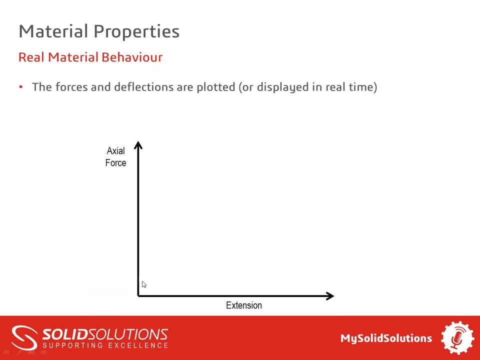 measure this with a, with a ruler, for instance. I've got a. oh, the forces in deflection, the plotted or displayed in real time. so we measure the force and plot against deflection and if we're with, we're stretching a ductile material, that's a material which is able to stretch, then we expect the curve. 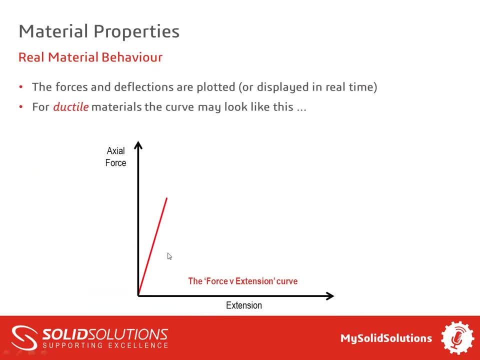 to look something like this: initially it will have a or it may have a straight line. it's not necessary, can have straight line, but for steels it'll tend to have a straight line where there's a proportional relationship between the extension and the force. we will describe this region as being an elastic region. 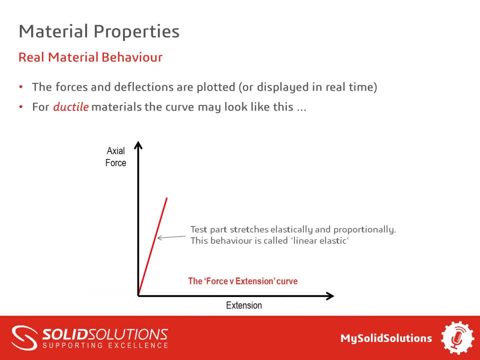 and a proportional region. it's elastic because if we release the force and the specimen will just spring back to its original shape, with no permanent defamation, because this is a straight line. in this particular case, we call this a linear, elastic defamation. at some point the material will begin to. 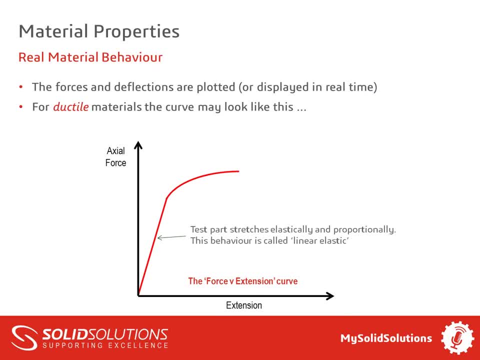 fail and we'll reach a yield point where we are no longer in a linear relationship and we get a much larger extension, so we have a large strain, so we get a change in behavior and then we get a region which is no longer proportional, so it's no longer linear. we're now into what we term a nonlinear. 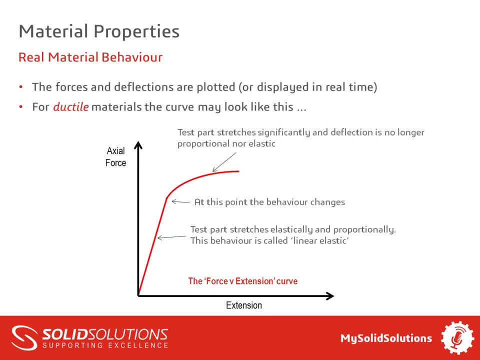 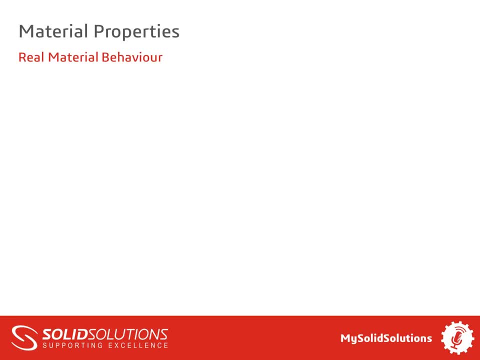 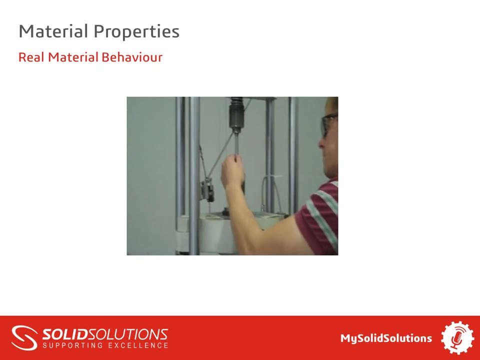 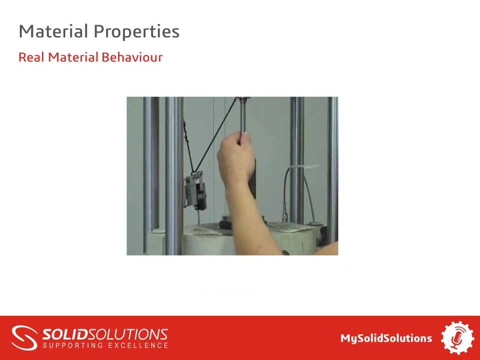 region and the material is no longer elastic, which means it will then take a permanent defamation if we release the load. now I've got a little video here. I'm hoping you can see this. it's one of one of these machines being used in practice. the video might be a little bit jerky just because of the 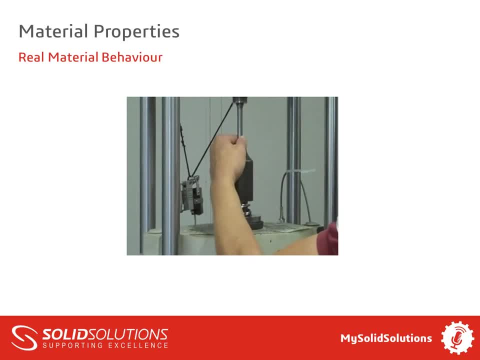 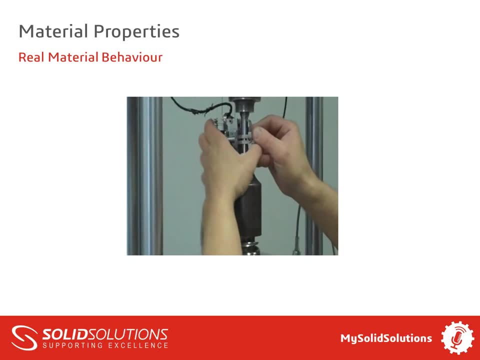 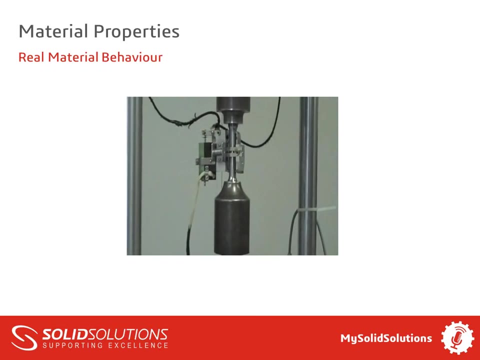 bandwidth on the internet, but you'll, you'll feel, I think you'll see enough to see what's happening. so the jaws, the specimen's been loading the jaws, the, the guys are putting in an extensometer which will measure the deflection and you'll see in a moment, as we 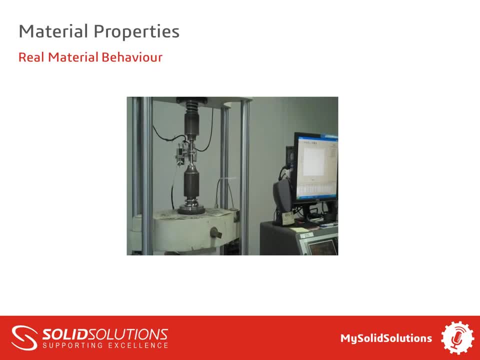 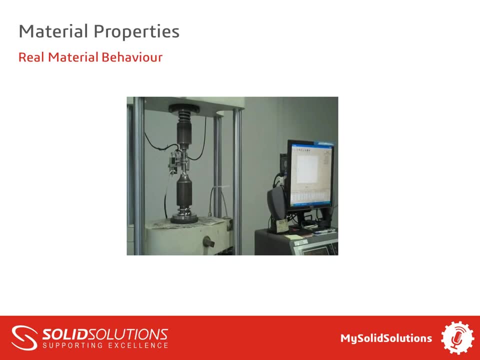 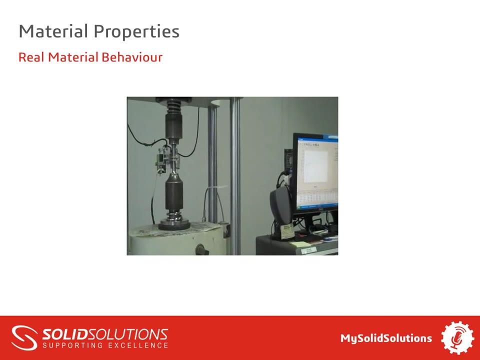 run out. there's a computer on the right hand side and there's a graph being which is going to be automatically calculated through the electronics and the machine's going to stretch this. and if you just look at the graphs now, you can see that the little line appearing is no suddenly beginning to become a horizontal, and we 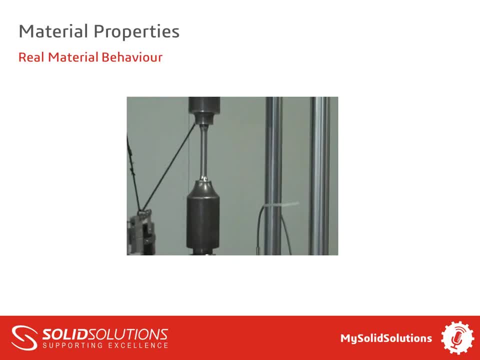 reached the, the yield stress, so you see that it doesn't look like anything's happened. but we have now actually yielded that material it's. it's strain will still be relatively small. its defamation will be small, but now it will have received a permanent set of permanent defamation. it's now being 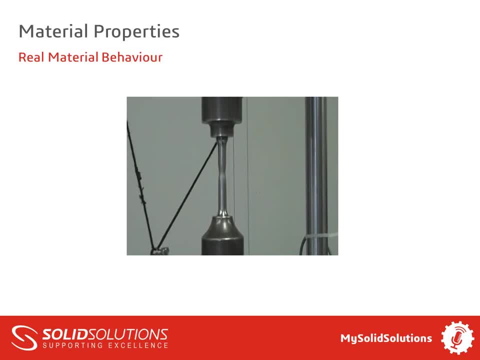 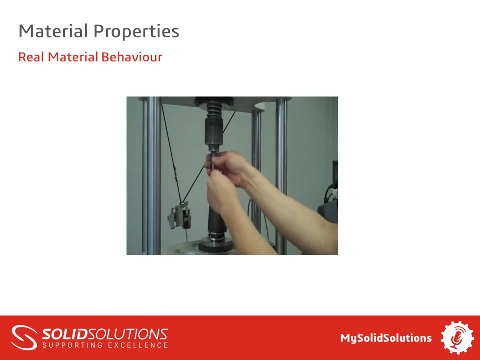 loaded again and you can say: now we've got a massive defamation, large strain it's being to neck. the necking is when we have large plastic defamation and ultimately it's going to break. and there it goes. this is a classic ductile failure. it's ductile because 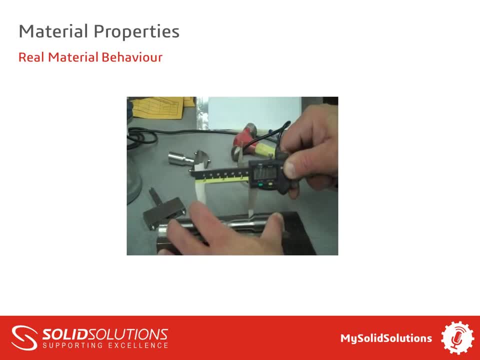 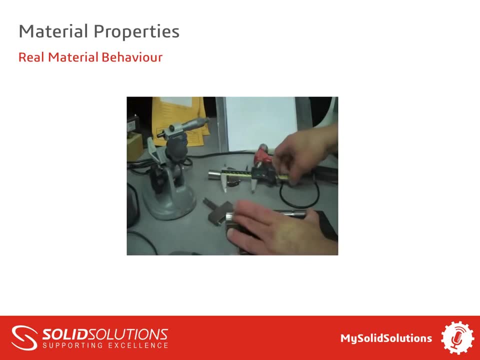 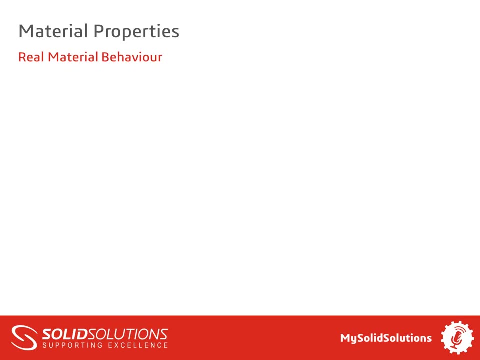 the material is allowed to, the material will stretch considerably before it finally fails. typically would then measure the overall extension and would also put a caliper across the width to look at the the width of the of the breakage point. so that was a ductile material and it stretched considerably. 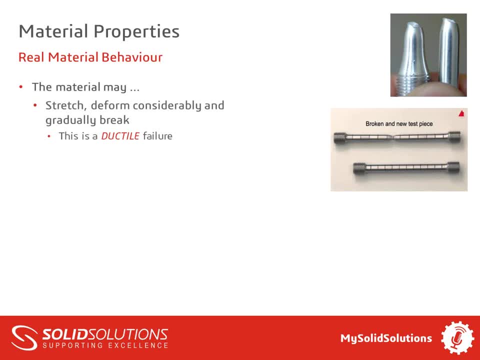 and if and it slowly and gradually broke. the way it breaks actually is along a 45 degree shear plane. and for those of you, look with us, last week we looked at principal stresses and principal stresses- in this case it would be a bigger maximum on a 45 degree shear plane and it failed when those 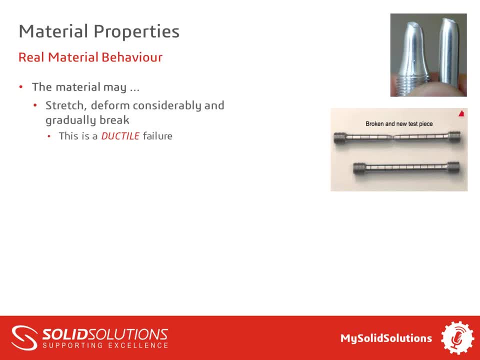 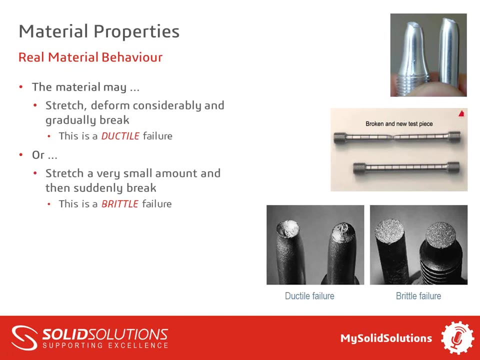 principal stresses. it caused the material to fail. you can actually see the the kind of necking and the 45 degree lines coming in here, so that's a good example of a ductile failure. if we'd put a different material in the machine it would have been not so interesting to watch, because it would 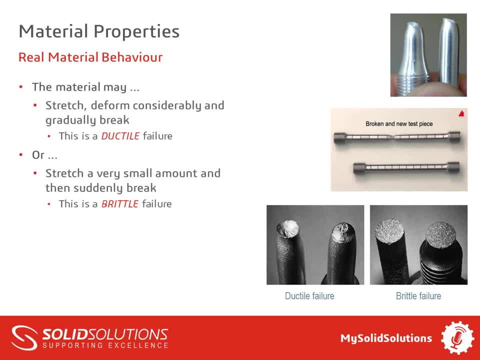 have just done nothing and then suddenly snapped and that would have been a brittle failure. and I've put some images here to show the difference between a classic ductile failure and a classic brittle failure. you can see the brittle failure: it doesn't have the necking and it doesn't have those 45 degree shear. 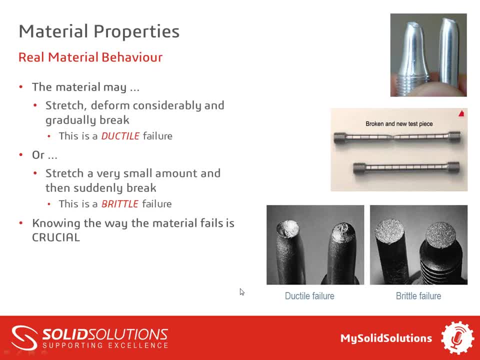 planes, you don't get the kind of cup shape. that's the point of failure. and my point here is that it's crucial to know how your material is going to fail. and it's crucial because if you apply the stresses in the wrong way, then you'll predict the wrong failure point. so we 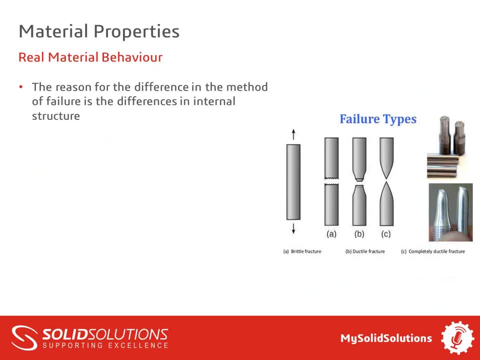 must treat brittle materials and ductile materials differently. you might say: well, why do materials behave differently in ductile materials compared to brittle materials? and it all comes down to the internal structure. whether it's a metal or a polymer, the internal structure will be different. a polymer has multiple chains and those that can slide across each. 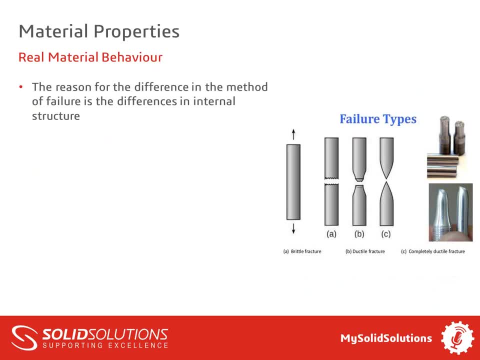 other. in a metal, the internal metallurgical structure for ductile material will allow some sliding, so the material can slip and slide and then deform before it breaks, whereas a brittle material, the material bonds between the atoms of the metal or the material if it's. whatever the material is, if it's brittle, will be such that they will both slip. 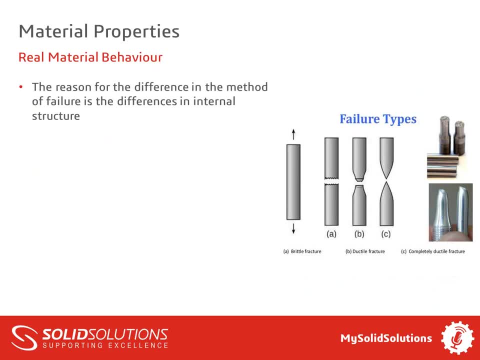 and slide and till, those bonds suddenly break catastrophically and typically they would. they break across a perpendicular axis, now perpendicular to the direction of pull. so ductile materials allow some sliding, brittle materials and have structures that prevent the sliding and then just fail suddenly. I would say probably the majority of materials we 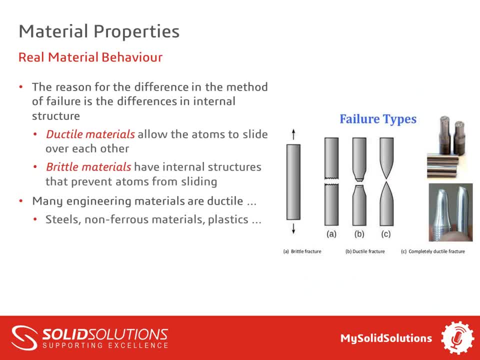 use in engineering are ductile materials, so steels typically will be ductile. plastics will be ductile in most situations. there can be situations where they're brittle: aluminium, copper, brass, for instance. they will all be ductile materials. some engineering materials are brittle, so some cast irons will be. 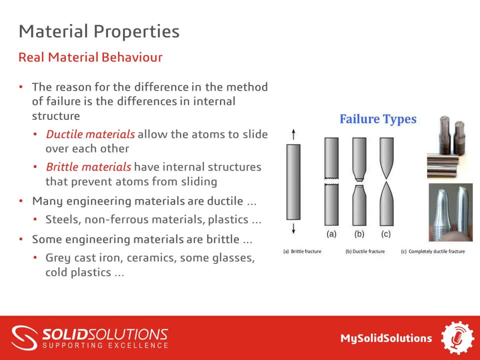 brittle ceramics will tend to be brittle, glasses can be brittle. cast iron is an interesting one because it can be both brittle and ductile, depending how it's being treated. there's types of of cast iron which can be ductile, so a spheroidal graphite cast iron. 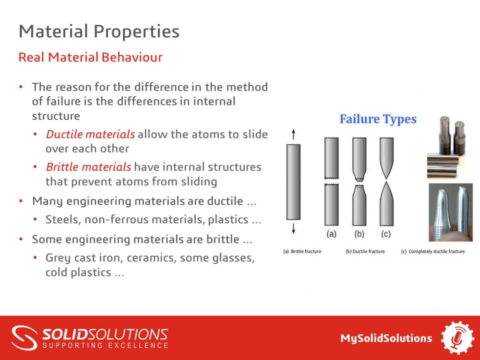 it's a bit of a one to get your mouth around. a spheroidal graphite is treated so that the the things which make cast iron brittle are kind of, which is the kind of graphite inside the structure. they are treated, heat treated, and they therefore don't cause a brittle face. 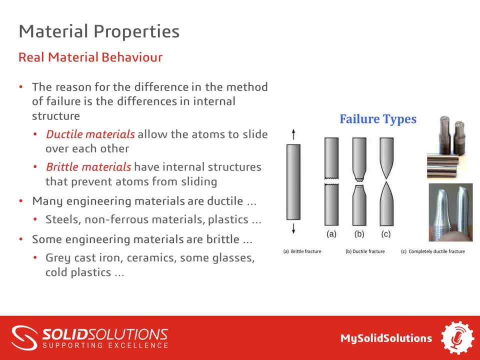 failure. plastics can be both brittle and ductile. if a plastic gets very cold, it can go beneath the brittle transition temperature and then it will behave as a brittle material rather than a ductile material. so materials actually get complex and you need to understand the material which you are using in your structures if you are not going to make some mistakes. 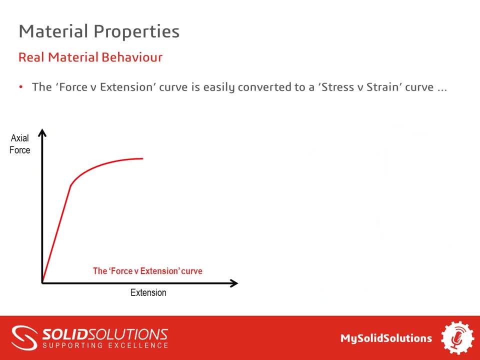 what I have shown you so far is how you would use a tensometer to create the force versus extension curve. that is what we can see on that machine: an axial force against extension graph, which might look like this: and then it is a simple matter to turn that into the. 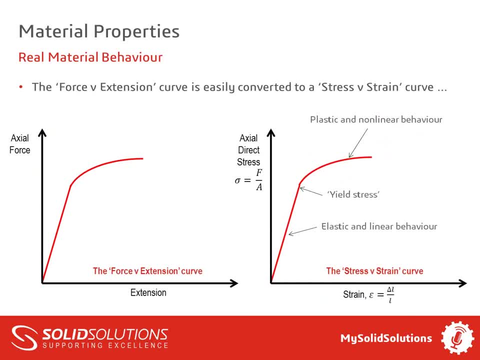 stress strain curve, we will know the area, the cross sectional area of our test specimen, so from that we can calculate the direct stress. and if we know the original length of our specimen when we stretch it, we can work out strain. So our force extension curve becomes the stress strain curve and stress strain curves. 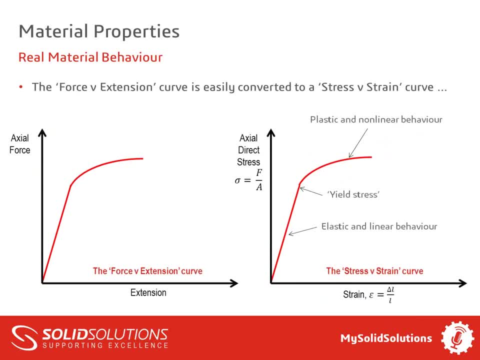 are really, really useful for all sorts of reasons. one reason is we can determine immediately whether our material has a linear behaviour or a non-linear behaviour. linear simply means that at least some part of it will be described by a straight line. so this red line here is. 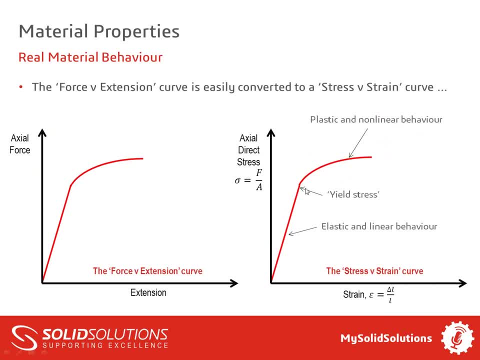 our linear, elastic region and at the end of our linear region we have a straight line. we will then get this onset of plastic Nigeria, a non-linear behaviour, and at that point, or very close to that point, we can define the yield stress, which is a fundamentally important material property. it doesn't always occur, unfortunately, some. 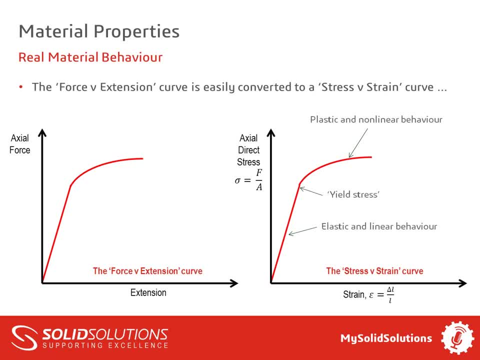 materials don't have a nice straight line. there is therefore no clear yield stress. if you have used solar吸imulation and you looked at some of the plastics, you might see that yield stress isn't defined in SOLIDWORKS. you might think that's a bit lazy, surely? 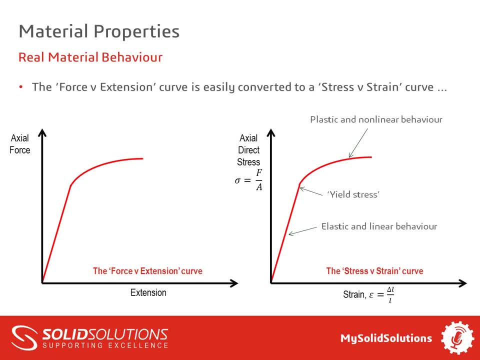 they could put that in. well, they don't. when there is in some sort of that, when there's a material which doesn't have a clear yield stress, it'd be wrong for them to do that because that would be defining something which is not clearly defined. for steels, we normally will have a yield stress because it will have a 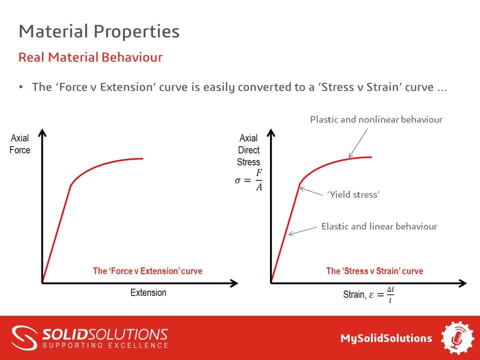 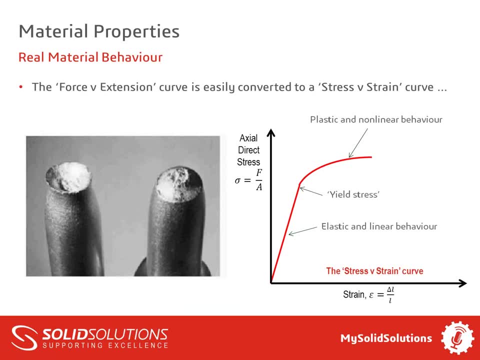 clear point where it begins to turn from an elastic material to a plastic material and there's a clearly fine yield. and there's just another shot of that cup where this would have exceeded the yield. in fact, all the stresses in and around this cup region would have been right up here at the top of our stress-strain. 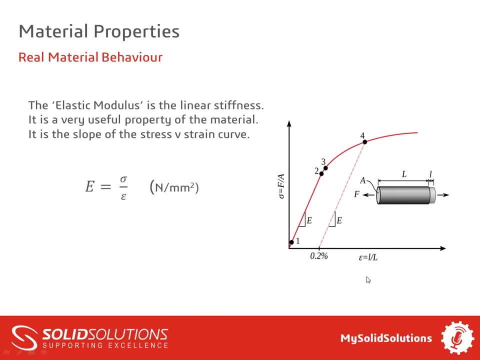 curve. now, having attained the stress-strain curve, we can then go on and deduce the elastic modulus, and we do that because it's simply the slope of the stress-strain curve at any point. so we take the stress ordered the, or we work out this: look at the slope of the stress-strain curve by dividing the: 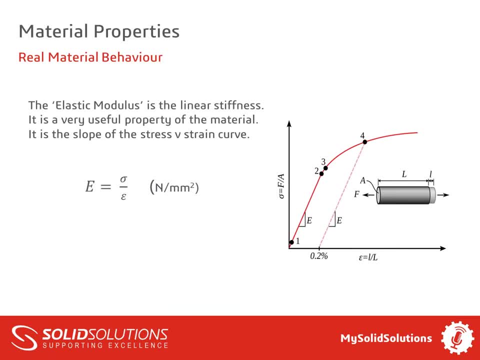 stress into the strain at any particular point that will become the elastic modulus. strain is dimensionless, so the units take on the units of stress, which is Newton's per meter squared or Newton's per millimeter squared. this will typically be a big number. it's usually 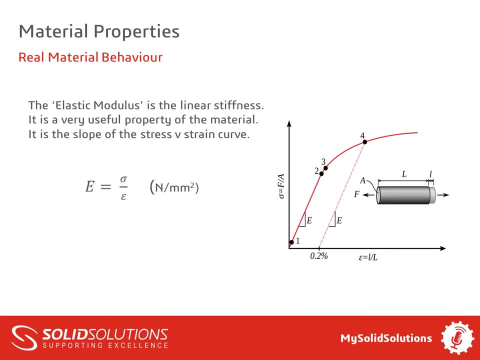 expressed in giga Pascal's, which is thousands of alright for any line, these of megapascals, or times 10 to the 9 for giga, and it's very, very important properties, effectively, this stiffness. as I said earlier, this is also Young's modulus, it's the same thing. 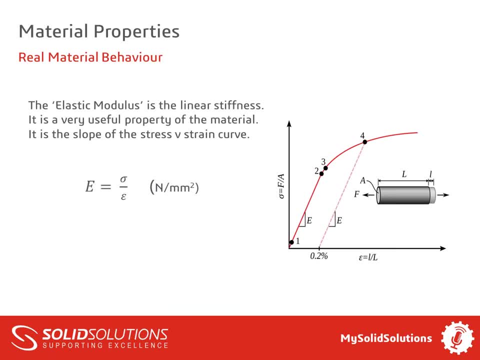 sometimes there is no clear yield point, so there's no clear yield stress, and so therefore we have to or we can. if we choose to define a yield stress using a different method- and this is a typical solution- we can define what called proof stress. that simply means that we mark off, not point, a value in our strain, and 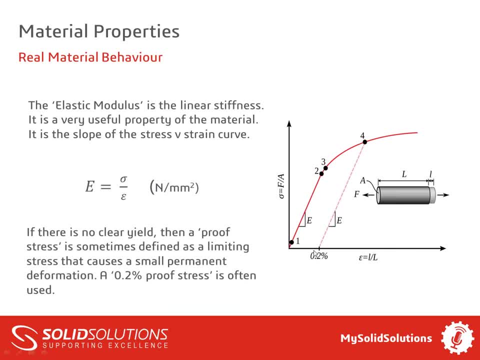 not point two is a commonly used value. so we mark off not point two. we then take a parallel line to the linear region and we mark off point four up here and would you define that as being kind of the the yield stir or the stress at not point two percent strain? so 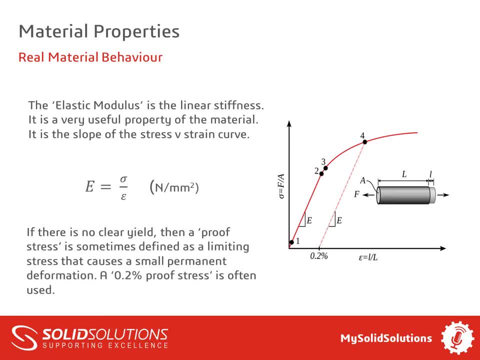 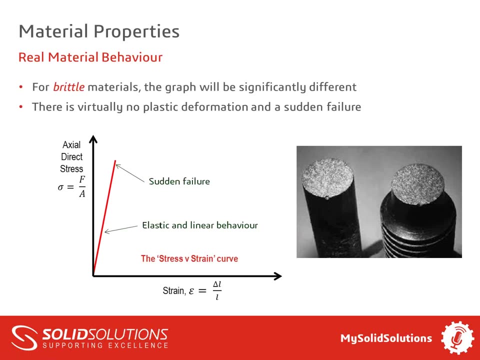 it's called a proof stress. we typically use this where we have a material which is doesn't have a clearly defined yield. so an aluminium might have a- not point two percent proof stress instance. so that's really are what I want to say, but it ductile materials. when come to brittle materials, the stress strain curve. 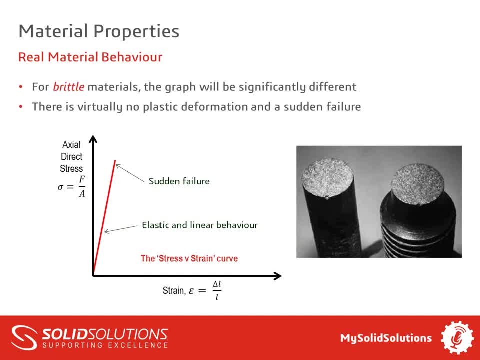 is much different. there is no curve at the top and this, say, linear portion will tend to be very, very steep. brittle materials tend to be very stiff and they will get to a point where they suddenly fail. you might see a small kind of a kick up here where you 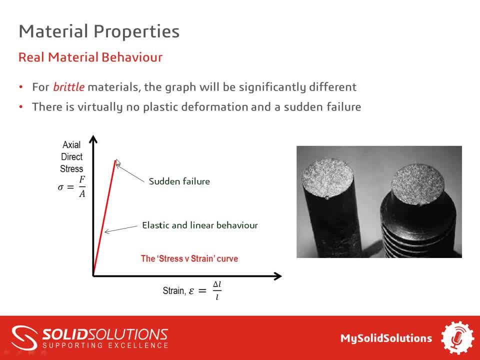 suddenly get a little curve at the end, but that's normally very small, and you get a sudden Onset of failure and the material will then split horizontally Due to the, the bonds in the metal or in the material just breaking down again. we can define an elastic and a. 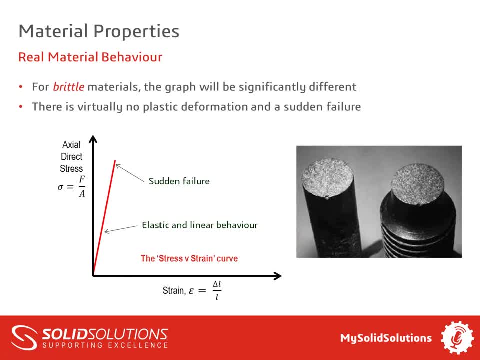 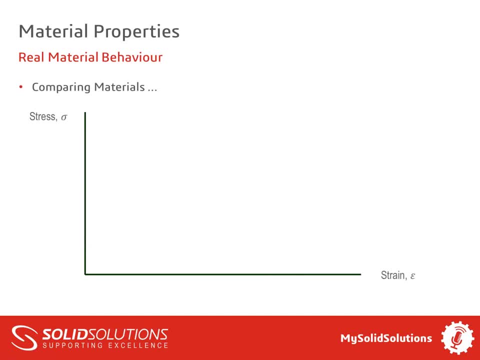 Region. we can define the Young's modulus of elastic modulus, as we did with ductile materials, you. So let's just compare Materials just kind of symbolically or graphically here. This is what a ductile material would look like. we'd expect to see a. 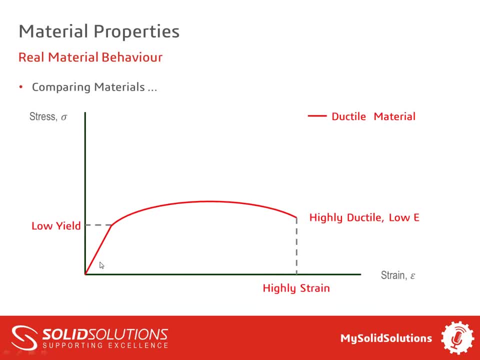 fairly shallow slope, therefore a lower stiffness and their lower elastic modulus, followed by a long strain region and high ductility. If we compare that with a British Material, will have a much steeper slope. typically We won't have a strain region or a high strain region, but it will suddenly fail at low strain. 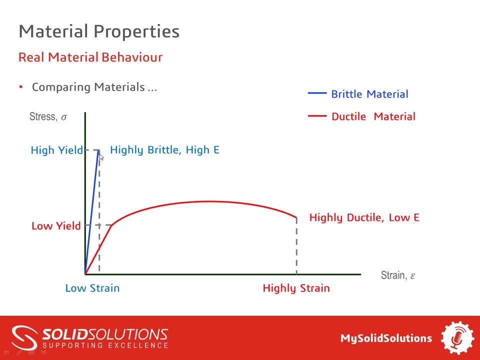 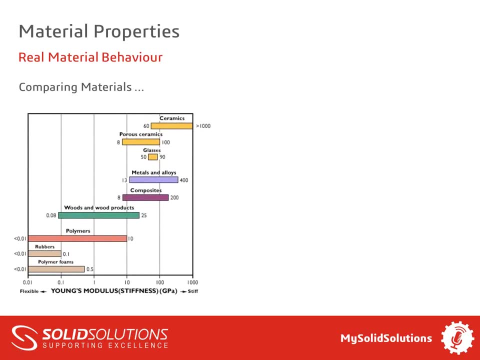 And we'll have a high yield stress. Just some graphs, so images off the internet. this is a comparison of Young's modulus for various materials. the scale on the bottom is in gigapascals and and When. if we look at the top right, we have ceramics which are very, very brittle, very, very stiff, and so pottery. 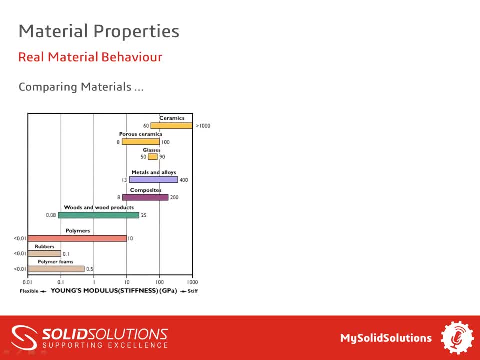 Brick, I will be ceramic type materials. They'll tend to be very stiff and when you apply load to them they won't strain very much at all. But suddenly crack and break. Now at the other end we've got rubbers. Rubbers are highly flexible. They will strain a large amount. 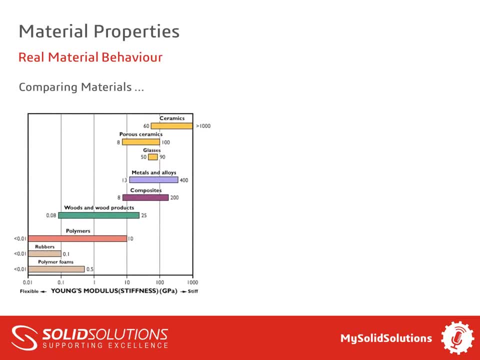 sometimes five, six hundred percent. So in other words they can stretch five, six hundred time five or six times their original length before they eventually fail. Metals will tend to be reasonably stiff, But not necessarily brittle. Here are some typical values. So we've got Young's modulus here expressing Newton per meter squared. so this is in. 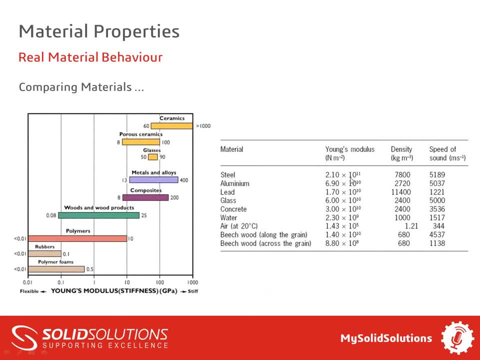 Gigapascals. sorry, in Pascals, so we've got the ten to the eleven here. so this is two hundred and ten thousand Thousand thousand Pascals, or two hundred and ten Thousand to Mega Pascals, or 210 Giga Pascals. 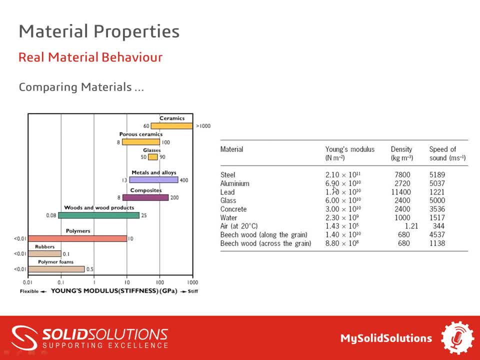 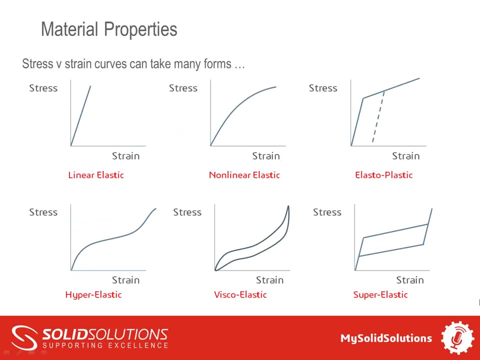 Notice that here, aluminium is just about a third as stiff as steel, And lead is only a fraction of stiff steel or Aluminium. Stress strain curves, though, may not necessarily be Linear ones. they may not have a straight portion, They may have all sorts of shapes. I've taken this from our nonlinear training course. 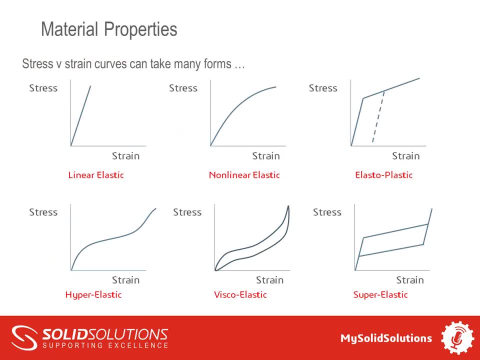 but shows the sorts of materials which you may encounter. This one here is a nonlinear elastic material. so it will have a. it won't have any straight line on the curve But it will be elastic. so if you release the load it will always come back to the origin. 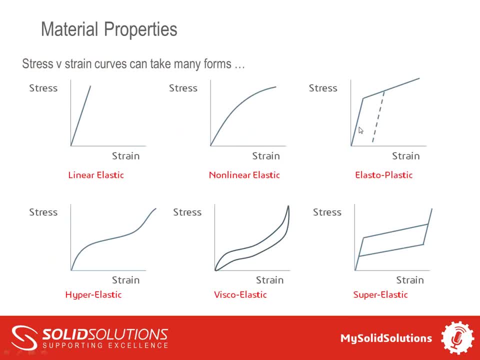 This is more typical of a metal where you would have a linear region followed by a plastic deformation, But it will be Have a permanent deformation if we release the load at this point above the dotted line, and When the load is released, Then we'll end up with a permanent strain represented by the end of this dotted line. 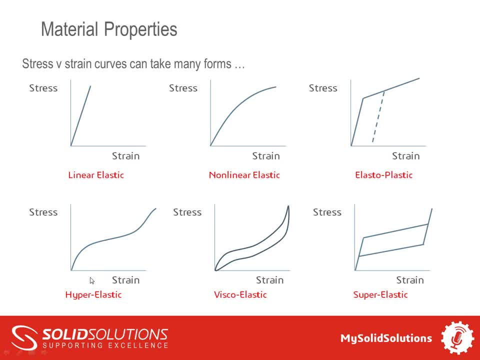 This one's what we call a hyper elastic, so this would be like a rubber. This would exhibit very large strains when you get this kind of s-shaped curve. Visco elastic would be a material which can actually flow. it remains in a viscous state, so glass would be an example of a viscous. 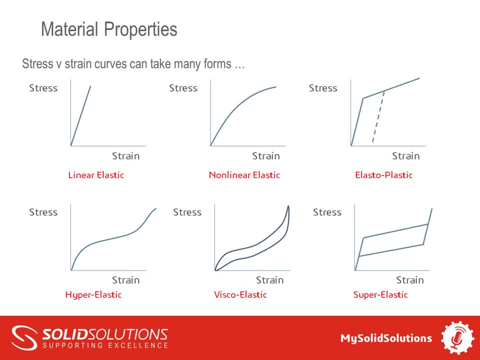 elastic material and It will Perform differently in loading and unloading. So as it so it's that it's kind of rates dependent, so if you apply the load quickly Or slowly, you get a different response. Finally, there's one down here called super elastic. This is a nickel, titanium type alloys. where you get, you get a different loading and unloading curve. 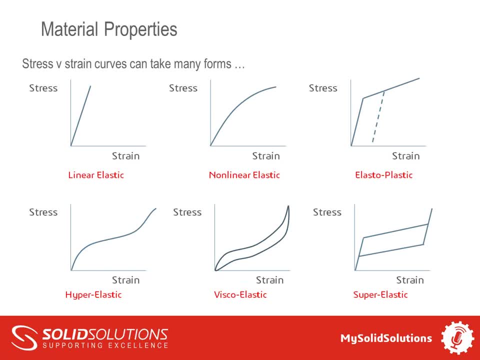 So I just put that in just to make you aware that materials can get quite complex in their stress. brain curves, Fortunately, many times when we're doing our calculations with dealing with elasto plastic materials where we're working in the linear range, So we're working at low stresses and low strains, where we can assume proportionality. 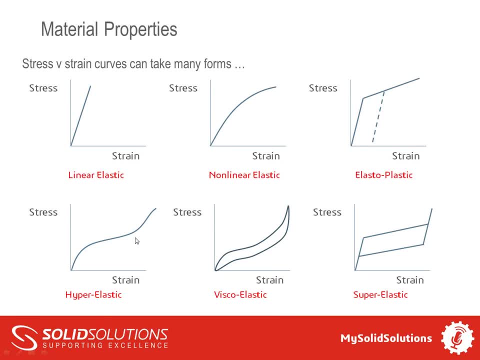 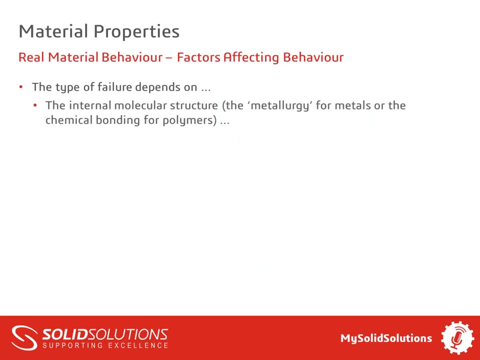 The. but the one to be careful with is rubber, of course, because rubber is hyper elastic, So it's very difficult to do hand calculations on rubber. What other factors can affect behavior? well, We've seen already that the internal molecular structure, Whether it's a Metal or whether it's a polymer, the internal structure, will affect the, the way the material behaves and how it, ultimately how it fails. 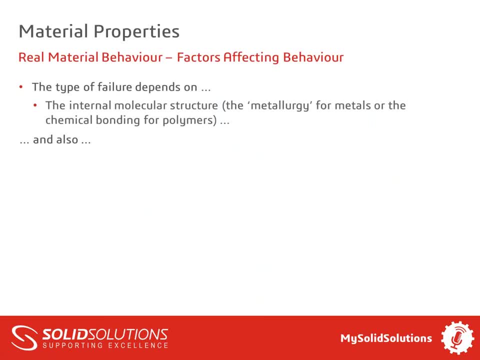 But also there's a range of other factors which you must also consider. temperature: Materials will behave differently at a higher temperature than a lower temperature. How the how the The material has been heat treated. if it's been heat treated. if it's a metal and it's been heat treated. 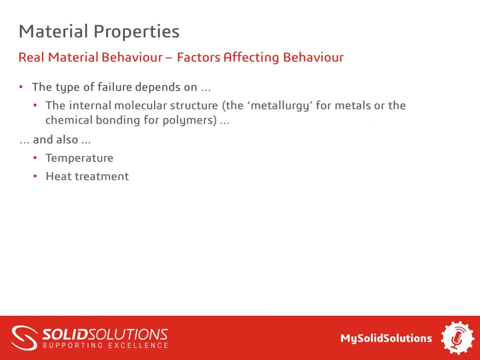 Then you can change the internal molecular structure, particularly if it's perhaps quenched to make it hard The environment- corrosion for instance- will affect the material behavior. Now the speed of force application. I alluded to that just now. with viscous materials They will perform differently with the speed at which you apply a load. 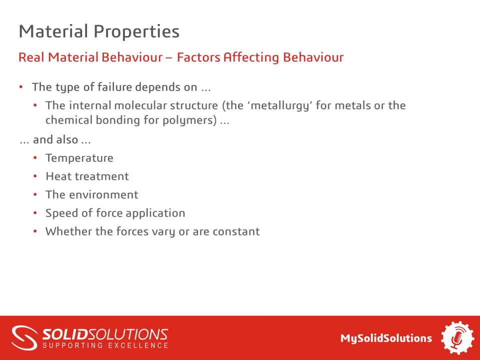 And if the forces are varying that will also affect the material behavior, behavior, particularly when we get into fatigue applications, The nature of the stress which we're calculating. something May behave differently in shear from the way it behaves in compression and tension rubbers in particular, Paved differently in in. 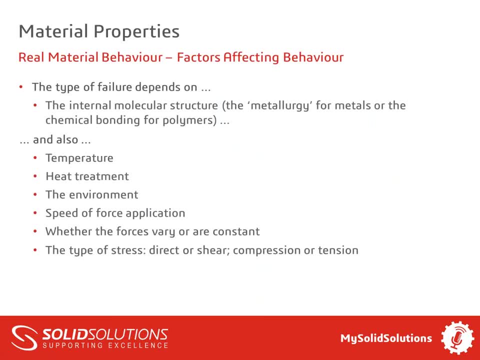 Uniaxial loading compared to in our planar loading, And also leaving the length of time that the load is applied will be. we'll be talking about this afternoon, And you may be familiar with a What we call a creep failure, Where a material subject to a constant load actually will fail, and after many hours, or sometimes over many years. 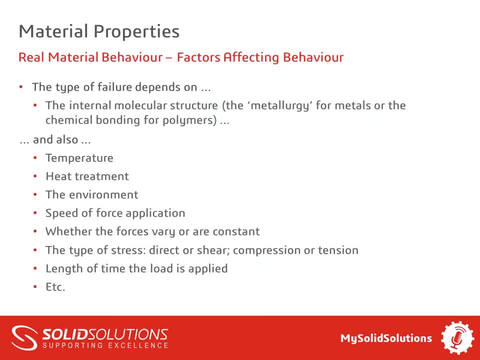 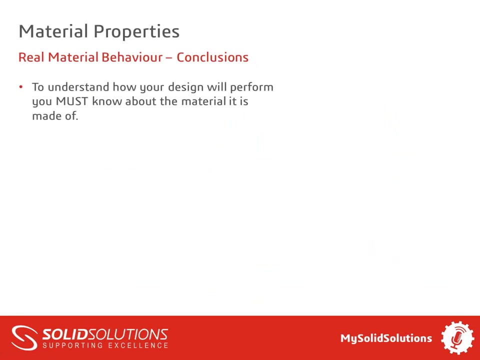 Simply because it creeps, And so on and so on. this isn't an exhaustive list. You need to read widely to Take of using to us an unusual material, to understand what other factors can affect your material. But see, these are some of the common ones, So let's just draw some conclusions now. to understand how your design will perform, you must know about the material is made of. 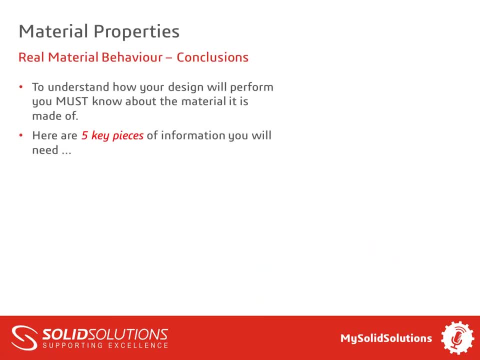 And here are five, five things I recommend you. you you try to find out as a minimum, and They can all pretty well be deduced from stress-strain curve, Which is why it's such an important piece of information. Firstly, understand whether the material is linear or nonlinear. 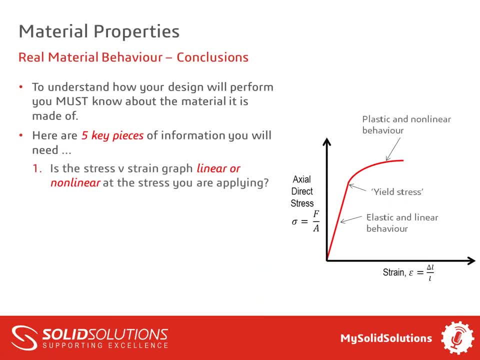 So that will affect how you do your calculations and it will tell you how the material will behave as the load increases. Secondly, try to understand what the stiffness of the material is. The elastic modulus, that's the slope of the stress-strain curve, is with. we've already discussed 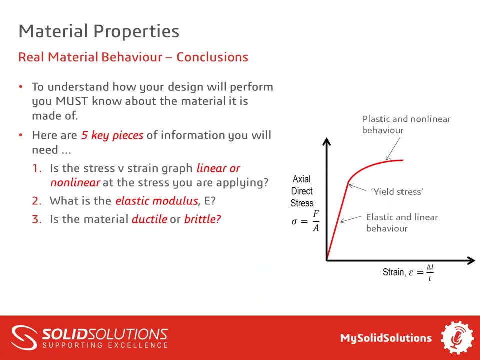 and Thirdly, and crucially, will the material fail in a brittle failure mode or a ductile failure mode? Fourthly, at what stress does the material break? if it's a brittle failure, what time, what temp? what Stress does it fracture? or if we've got a ductile material, at what stress does it yield? What is the yield? stress and 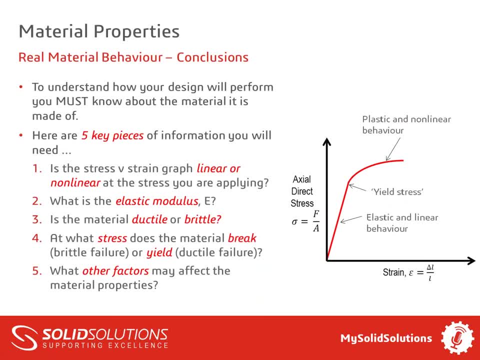 Finally, think about what other factors may affect the material properties. so this is a kind of a very brief overview on on Real materials and the types of properties you may need to understand or calculate or or, in fact, indeed in some cases, actually have tested for you, So that you can then go ahead and do your, your own engineering calculations. 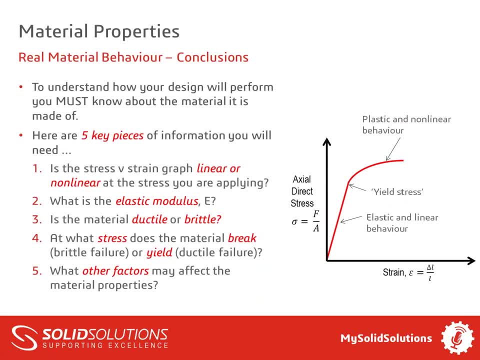 As I said at beginning, this is just a brief introduction, but would give you, hopefully, a an understanding what you might be taught on a undergraduate engineering degree program or, And if you want to understand more this, there is numerous YouTube videos, articles and, Indeed. you can do a whole spend our career in this. 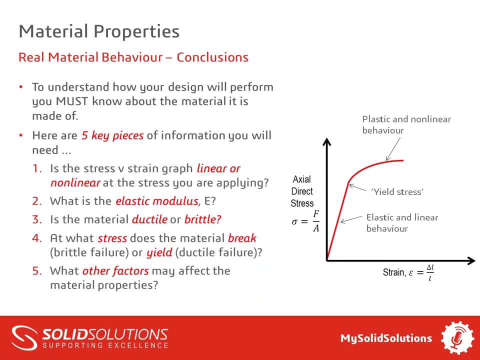 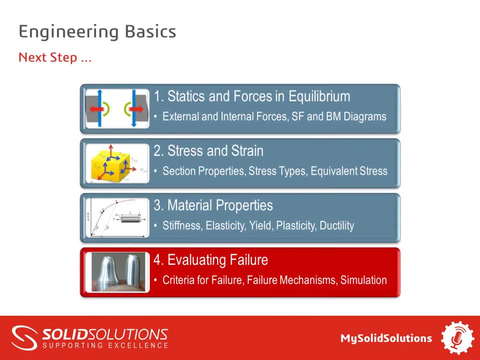 This area, but for those of us who are engineers or product designers, We need to understand these things if we're going to come to good conclusions about the, the way our designs behave. Next step, the final kind of piece of the chain, if you like, is then to say, okay, now we understand maybe something about. 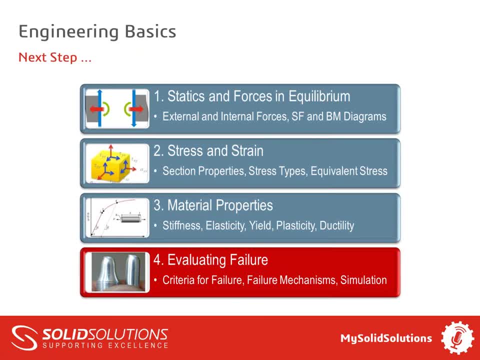 Forces, we understand something about stress and strain, we understand how our materials behave in the real world, and we understand things like stiffness and linearity and non-linearity. How can we then evaluate whether our particular Design is going to fail? and what we'll see is that there are a variety of failure mechanisms. 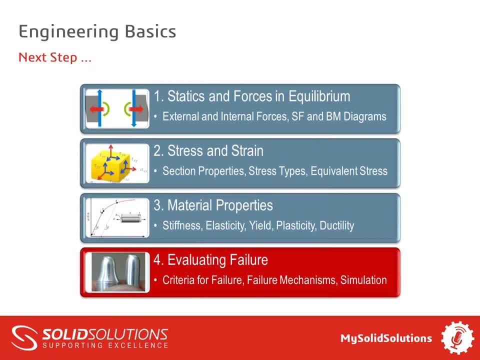 besides simple stress, and We need to be aware of those mechanisms and understand how are I the loading it applied. and finally, we'll touch on a little bit of simulation and Hopefully that will encourage you to look deeper at simulation. what we will find, what I find, is that 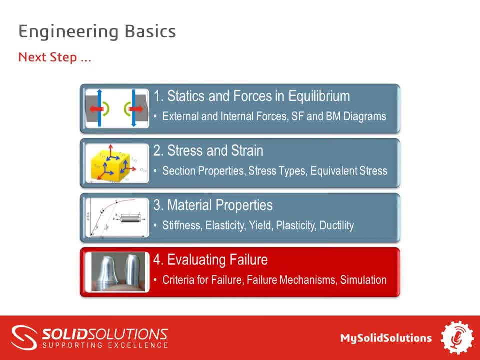 Hand calculations are great if you do them, but they're prone to mistakes. Simulations kind of take some of those mistakes away from us that we, you still need training, you still understand what you're doing, But simulation can, there, can, make things a lot simpler for us, and indeed simulation is often the only way of. 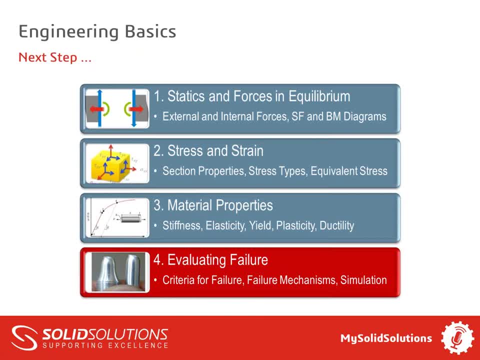 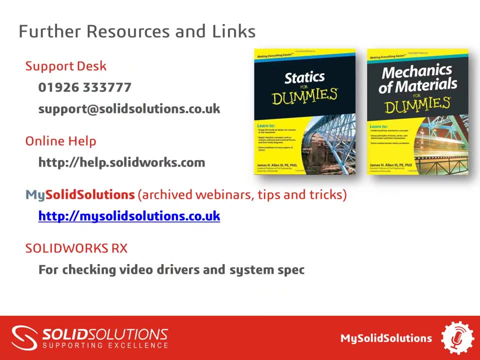 Working out whether a product will fail when we get into real complex parts and complex loading situations. There's our usual range of phone numbers and web cases that I've put those two Useful references up there as well for you. That's me done. Thanks for watching. I'll hand back to Nick now. 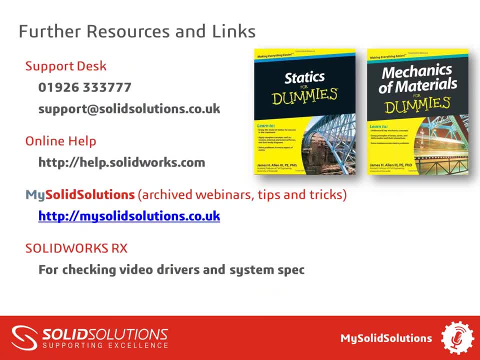 Excellent thanks, Andy. I felt like I spent the morning back in in university. that was a great insight there into engineering Materials. so, as I mentioned on screen are a few resources there that might be useful for you. This webcast will be uploaded to my solid solutions this afternoon. 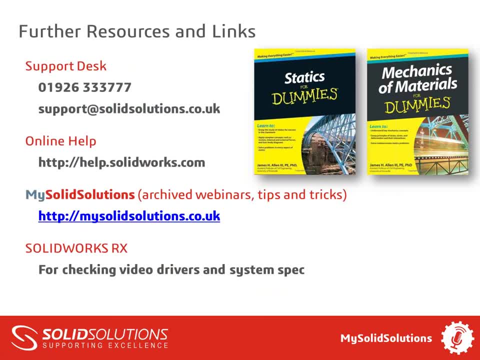 And you'll get a notification in 24 hours just to say that that's been uploaded successfully. If you do have any questions, we'll drop shortly into a Q&A session, but if you do need to leave, thanks for attending.